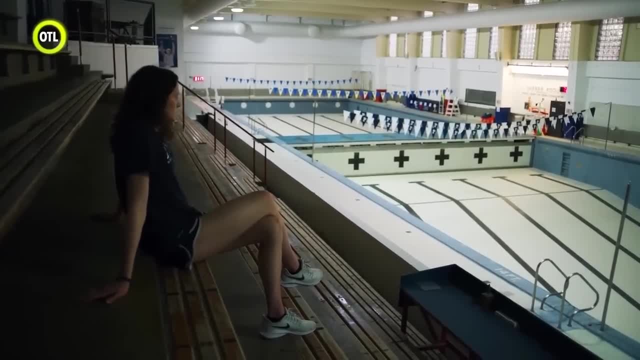 with suicidal thoughts. being trans is is not a choice I didn't have, and the other choices because not transitioning was not the end result of it. this was a crucial moment and I'm so grateful to have all this celebration in my personal life because I know it was the most beautiful thing i spent, thanks to you all today. you elq感谢. 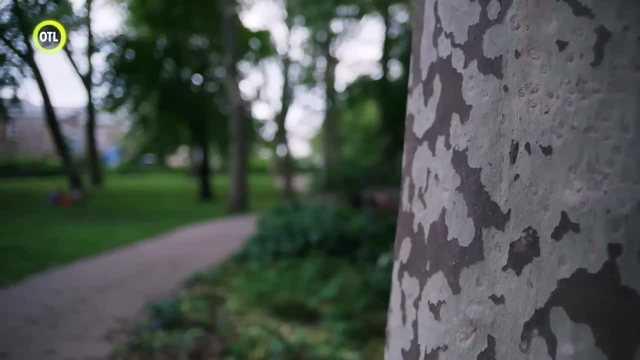 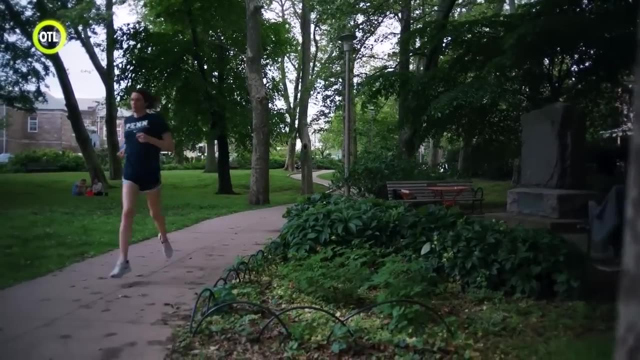 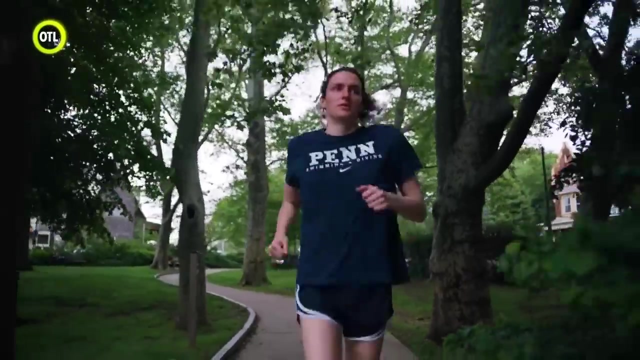 transcaretor best hands. an iyi phi waw to be to each and uh feels like being trans suo, drieта la dia, no il ii their sork西yi leading me anywhere. what are some of the changes that you experienced? I started hormone replacement therapy in May of 2019. one of the biggest was loss of muscle mass. I had a lot of fat redistribution, change sort of how my body looks and the shape. I shrunk actually probably about an inch in height. my feet got smaller- about half a shoe size or a full shoe size smaller now- and so it really does change your entire body. 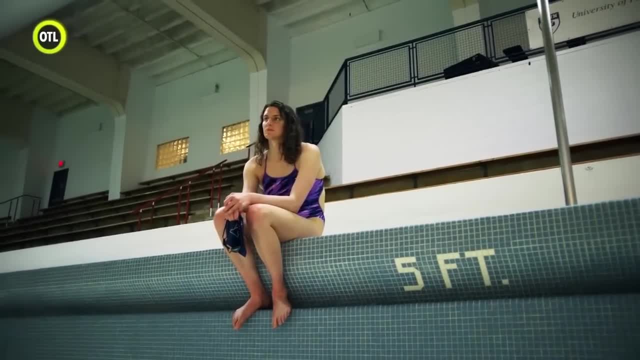 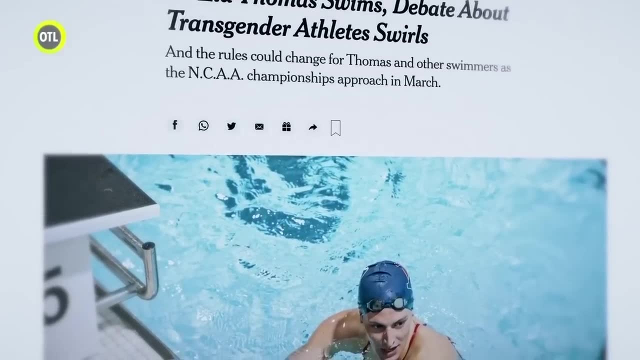 what reaction do you have toward other folks who feel that you shouldn't be able to do, that it's that you can't compete in the gym, you can't compete in the gym and they can't compete in the gym as well. and also as a result of this, like the 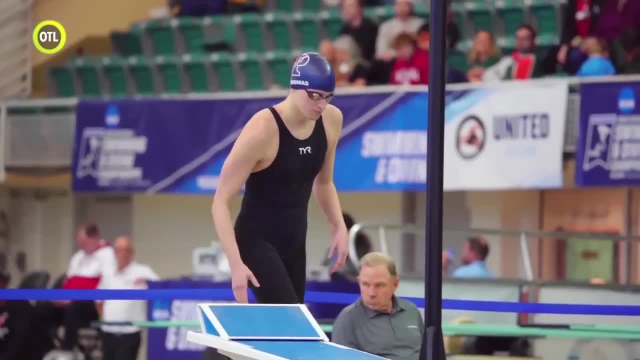 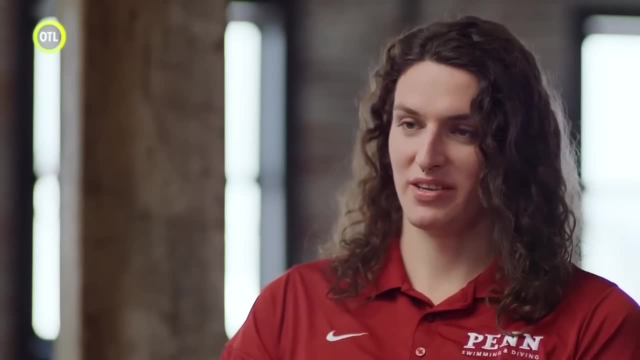 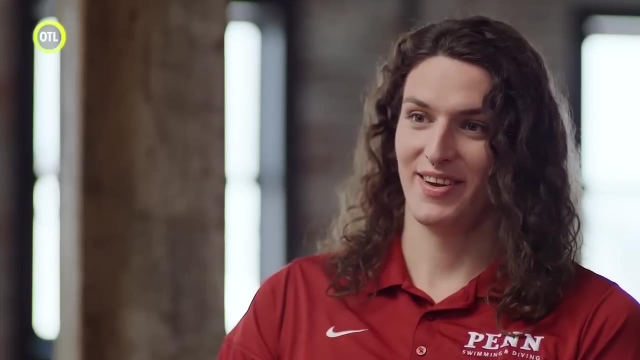 weight loss that I'm facing. I'm becoming less able to compete. trans women competing in women's sports does not threaten women's sports as a whole, because trans women are a very small minority of all athletes and the NCAA rules regarding trans women competing in women's sports have been 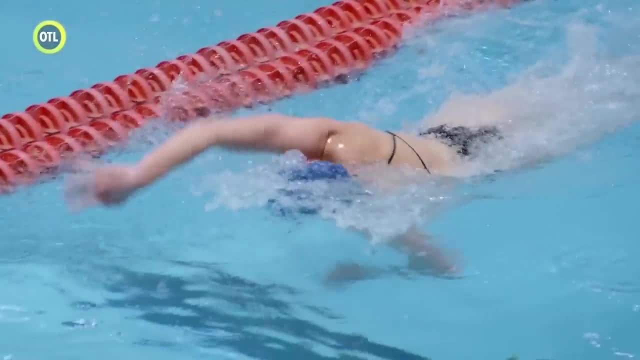 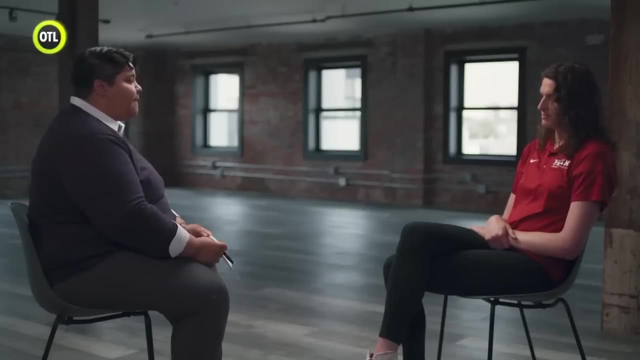 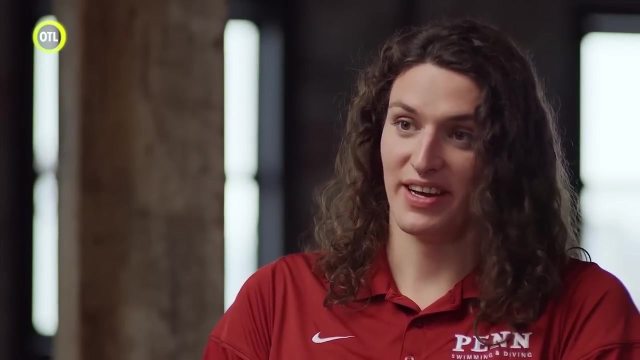 trans-women dominating. You know, through this experience for you, what's been some of your toughest moments. Some of the one of the toughest moments was when I first came out to coaches and to my team where I had no idea how they would react. 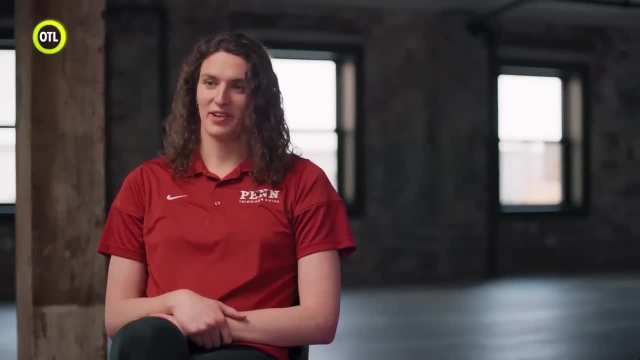 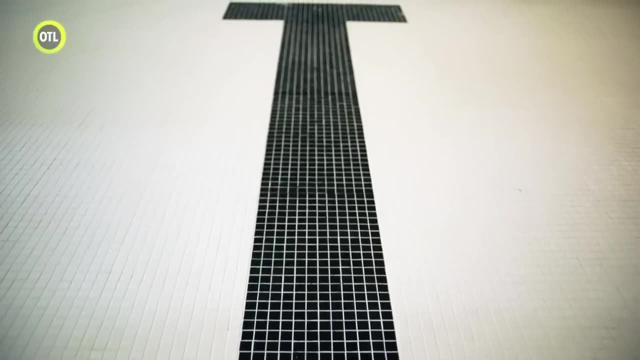 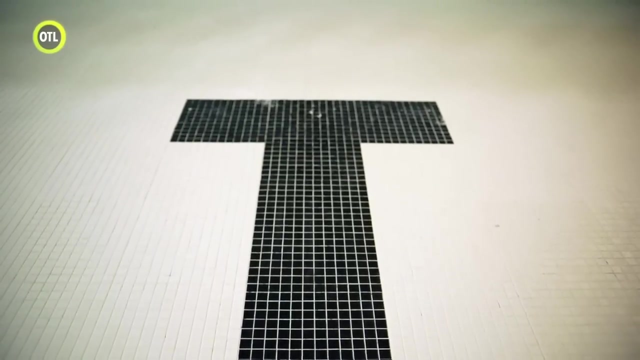 whether they would accept me or not And what the final outcome would be. It was sort of a leap of faith I had to take to continue swimming. I was very lucky to have supportive coaches and teammates And I went into my swimming career after that. 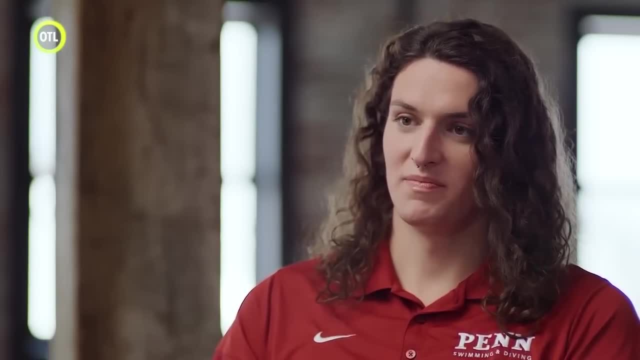 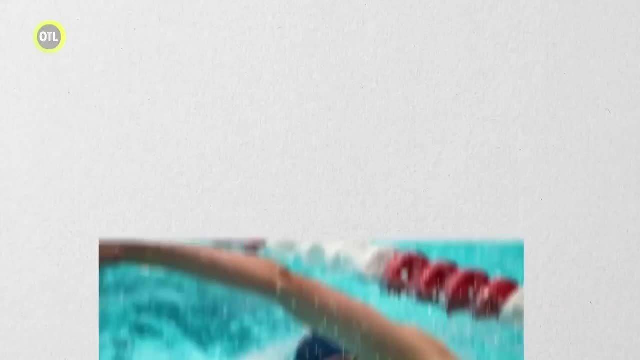 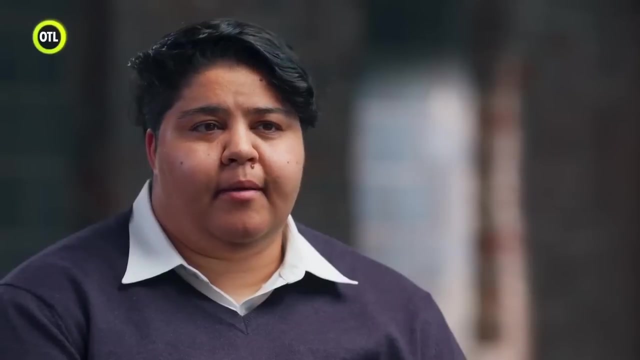 sort of not knowing what would happen. I didn't know how fast I would be. When you found out that a number of your teammates had anonymously signed a letter criticizing your participation, how did that make you feel? I knew there were some people who didn't support me. 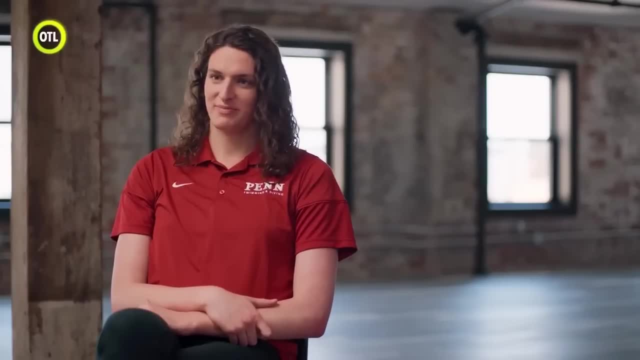 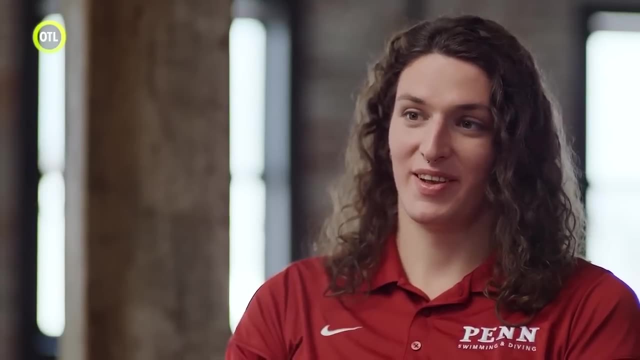 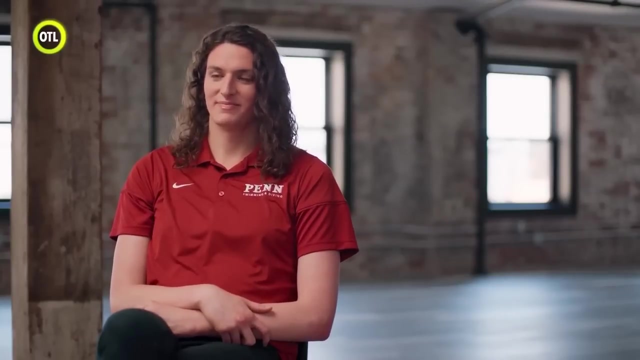 On a big team. not everybody is best friends with everybody, And I had my close group of friends And, as a more private person, that's all I needed was my immediate friends. I respect everybody on my team. We all had our issues. I respect everybody on my team. 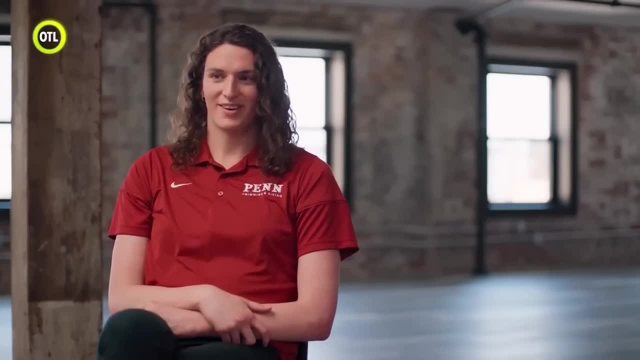 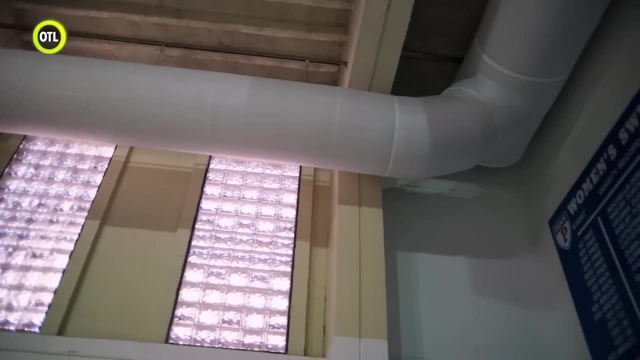 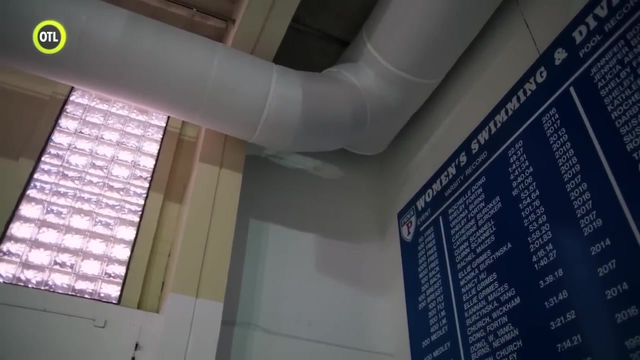 go through 20 hours of grueling work a week and I'll commit it to the sport and I won't harsh on anybody for that. On the record board in SharePool you still hold a pool record in your previous name. When you look at that board and you see that name, 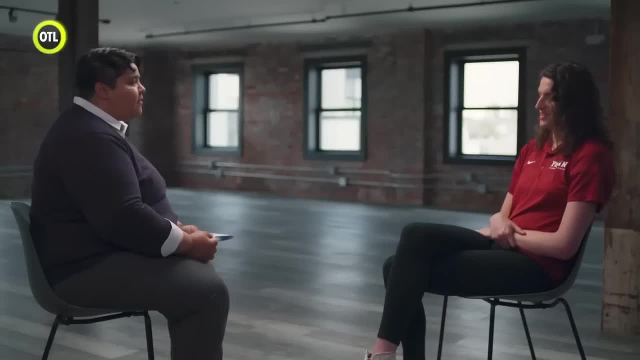 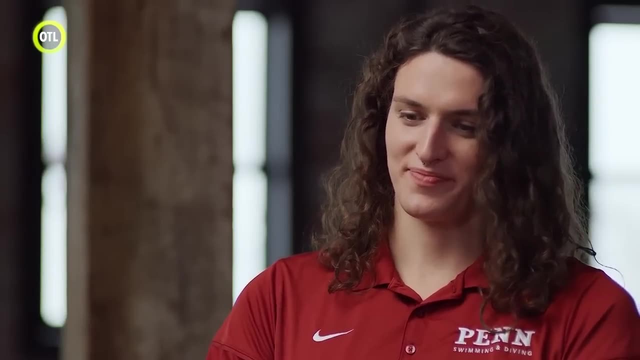 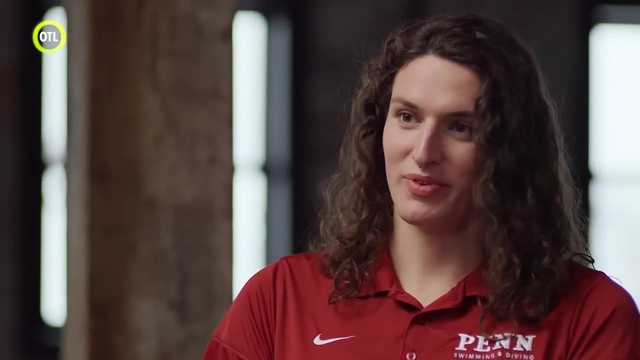 how do you feel about that? I, In a sense, I almost think of it as a different person, where It's sort of an interesting compartmentalization I have of my life pre-transition, where it is me and I'm the same person throughout. 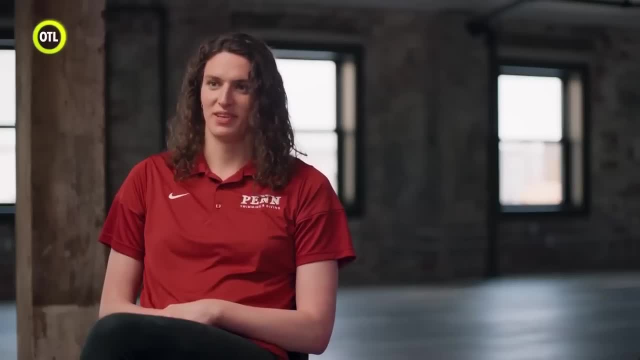 but in a sense it's like it's a different person And since coming out and transitioning, I've sort of rebuilt myself and who I am. so I just think of it. I just think of it as a different person almost. 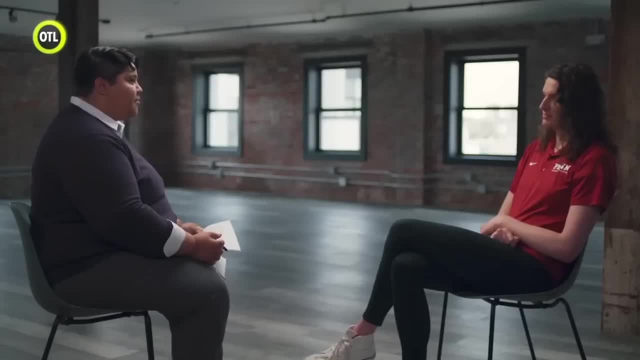 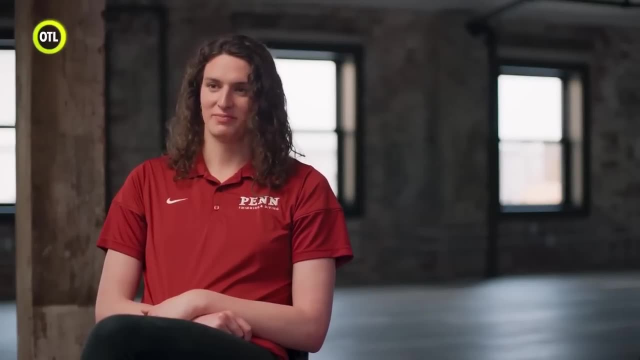 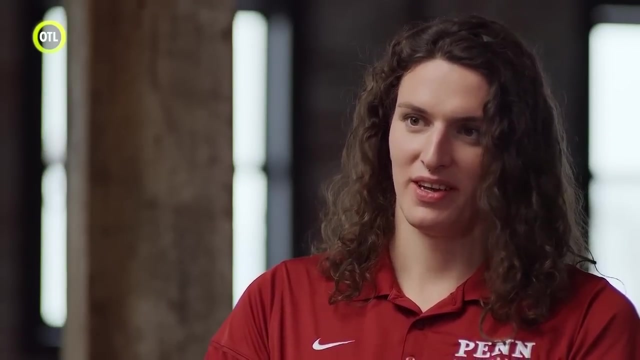 I asked you about your toughest moment, but what's been the best moment? My best moment is feeling at peace with who I am and it's coming home from a long day of school and swimming and relaxing and not worrying about how people will react. 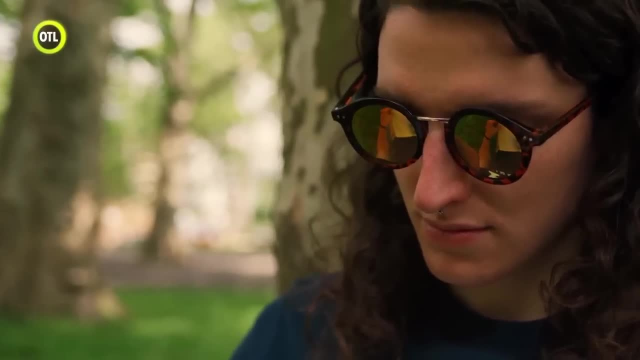 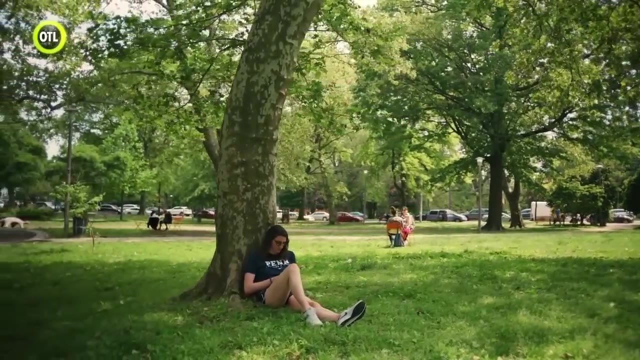 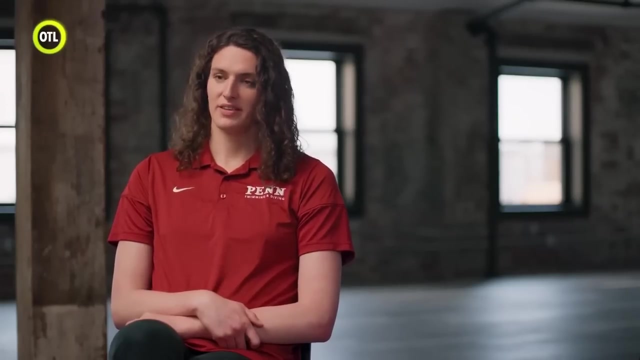 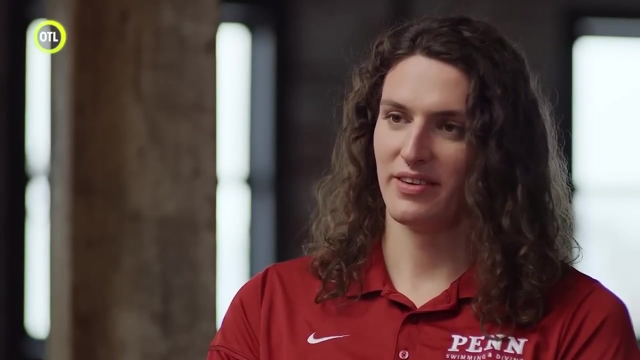 and not feeling the distress from gender dysphoria, and just feeling at peace with who I am. When you think of all you have endured in and out of the pool, was it worth it? I think, so. I would say yes, I've been able to do the sport that I love. 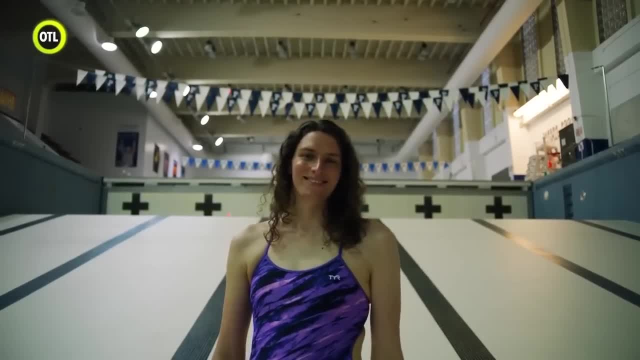 as my authentic self. The past has changed. I'm learning to be positive and learning to support others and my family- and my family is a family- And just to be content with it. You did so much for me, I'm so happy for you. And just also, I'm so sorry for you. I'll see you next time And that's all for today. Have a great day And remember give me a thumbs-up if you enjoyed this video and if you have any questions. let me know in the comments and I will come back to you with a new video or whatever message you want to send me.